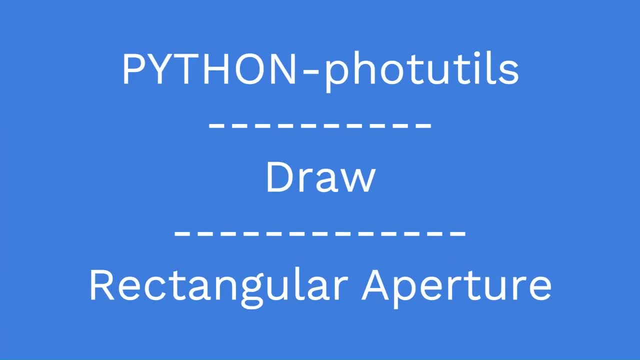 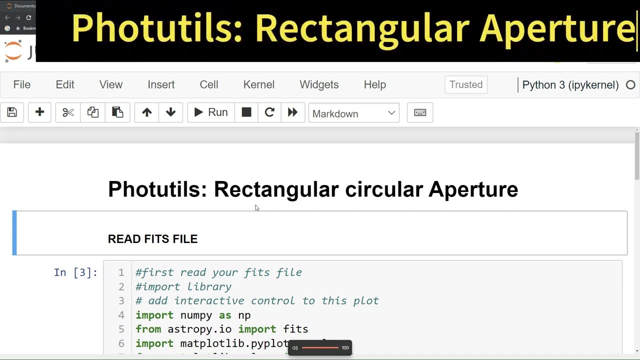 Hello guys, welcome to the CS Draw and in this tutorial we are going to learn about how to draw rectangular aperture around a star or a galaxy. Okay, so in earlier video we have seen that- how to draw circular aperture, So in this video we will be drawing rectangular. 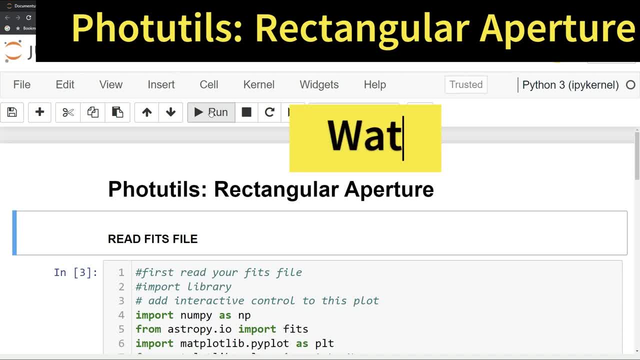 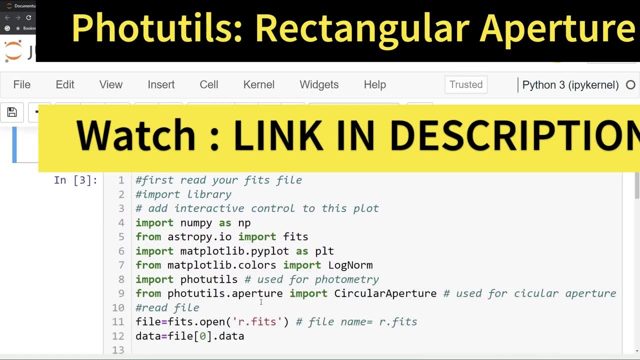 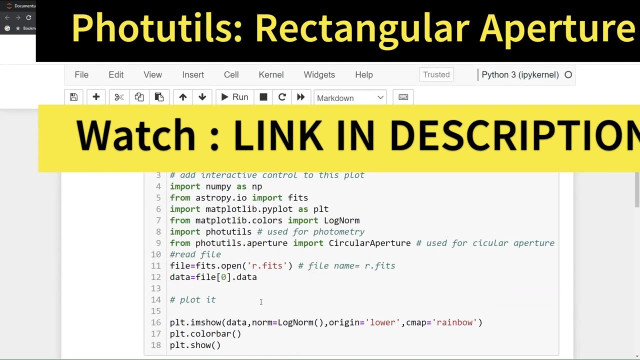 Okay, so for doing that you need to read your FITS file. So this is the code to read your FITS file and in our earlier circular aperture photometry we have known that how to read your FITS file and how to plot the image from the data. 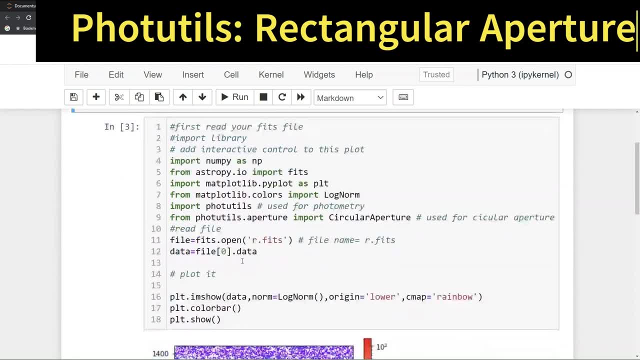 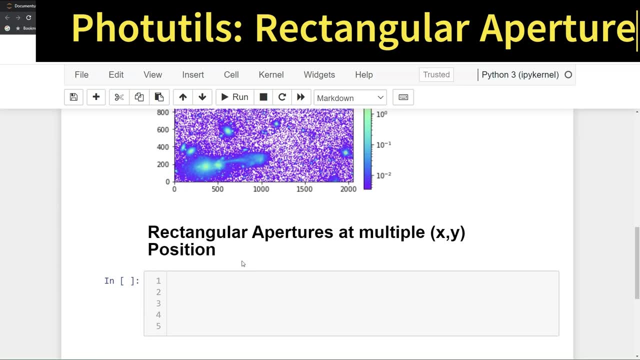 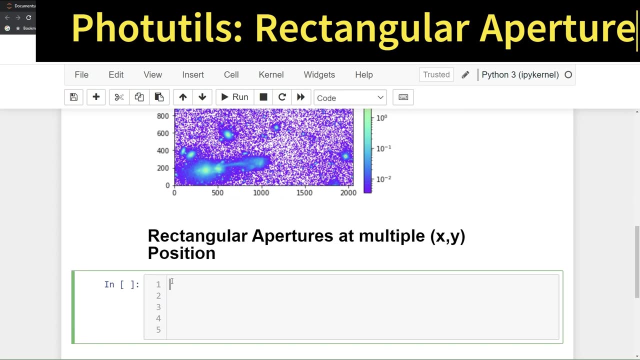 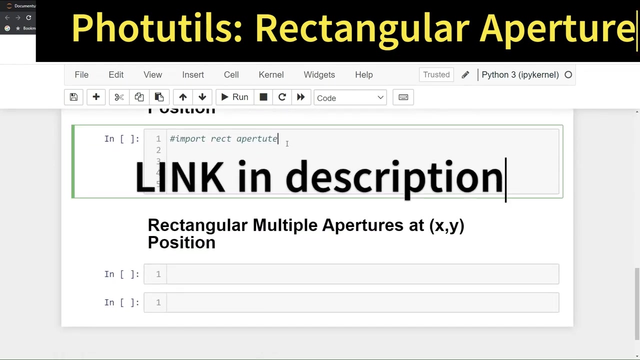 This is how the code looks like. You can always go back to my code and you can do the job from here. Okay so, now come to the rectangular aperture at multiple x-axis position. Okay so, Aperture- Okay So. 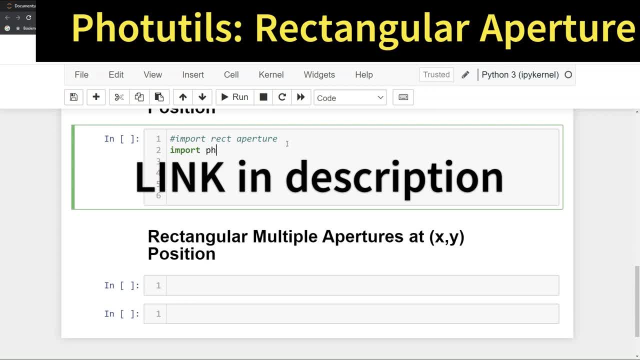 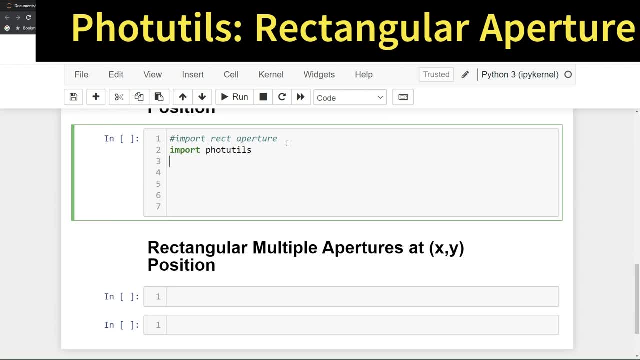 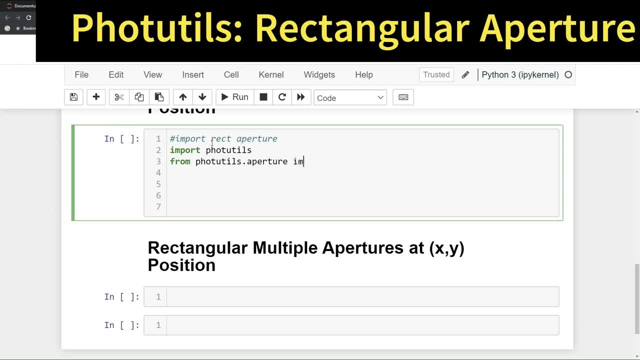 So you can do the same thing: Aperture: import a rectangular, a rectangular aperture. Okay So, this will do your job now. Okay so, now it's fine. So let me, let's look. Okay so. 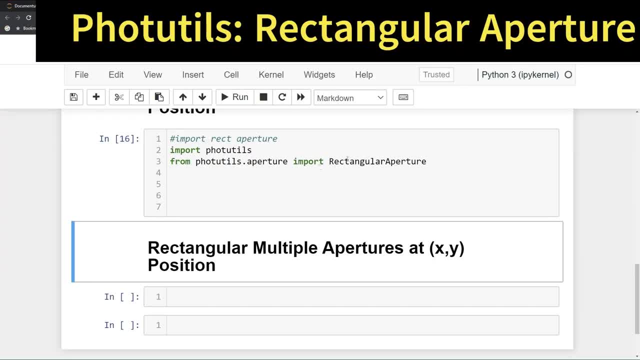 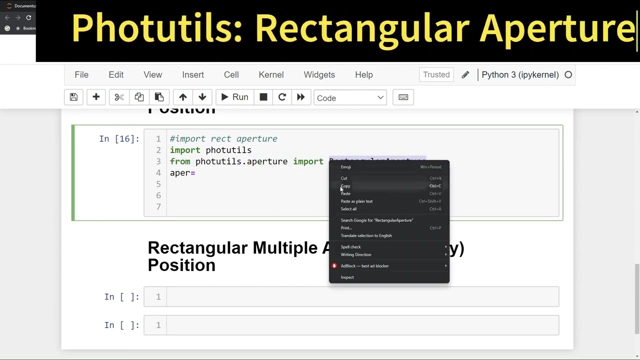 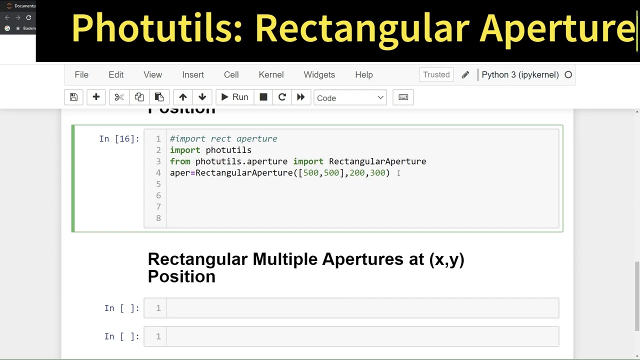 So, So, So, Okay. so now you want to draw a first aperture, Okay, so just type here aperture equal to and give, say rectangular, rectangular aperture, and give here your position, position and then width and height. You can also give theta, Okay, so you see it later. So for timing you can give position, So you can give, say you want to give at 500 and 500. Okay, and you want to give size, say 200 into 300. Okay, now you want to plot it. So this is your aperture. 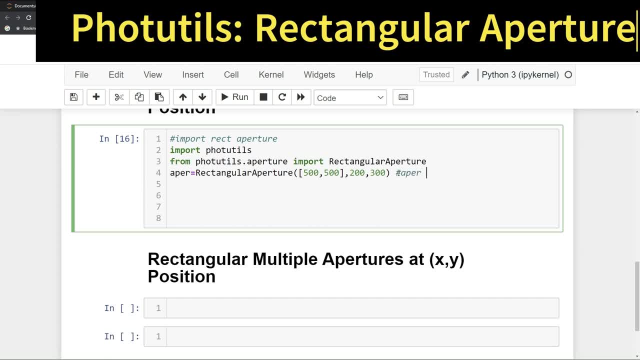 Aperture specification. Now you want to plot it. So for that type command aperture, dot, plot and you can give some color. So you can give, say, color, color equal to, you can give red and you can give line width equal to five. Now you need to. 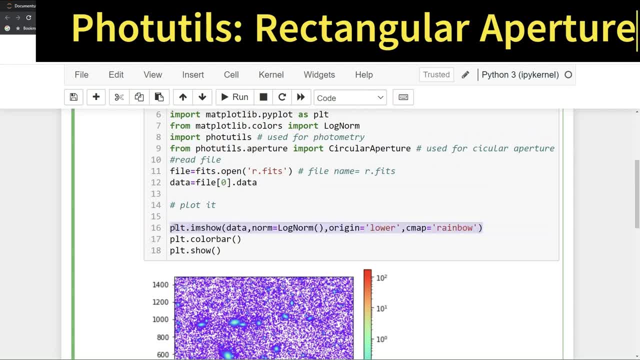 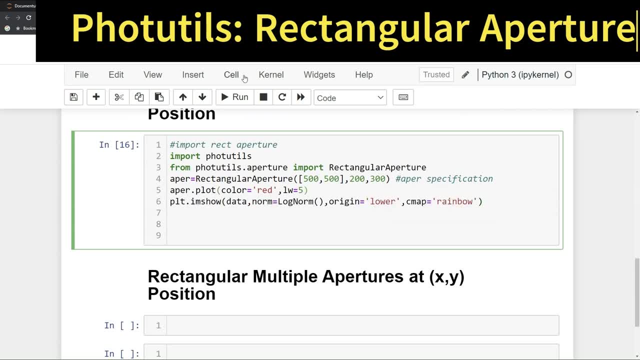 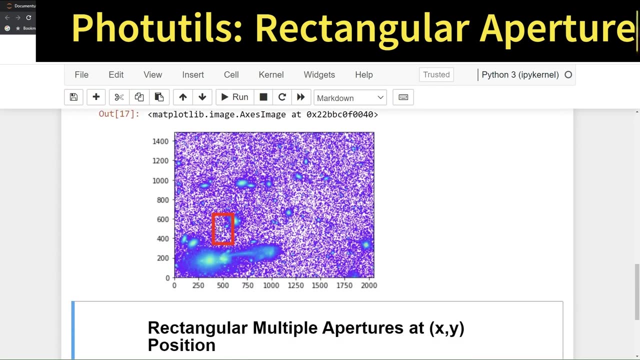 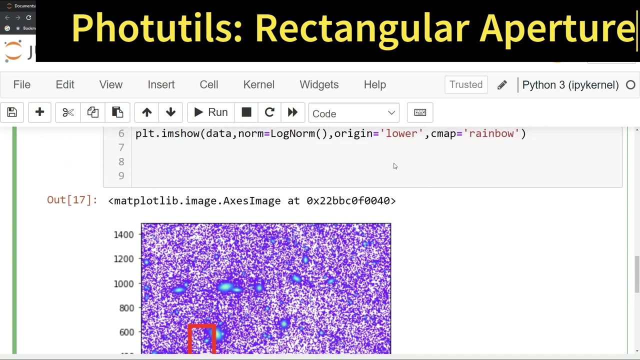 also plot the image above the image. Okay, so for that, copy this code here Now and run it. Okay, so here you can see that there is your rectangular aperture of this position and this size. You can also like increase the size if you want. You can make it say 500. 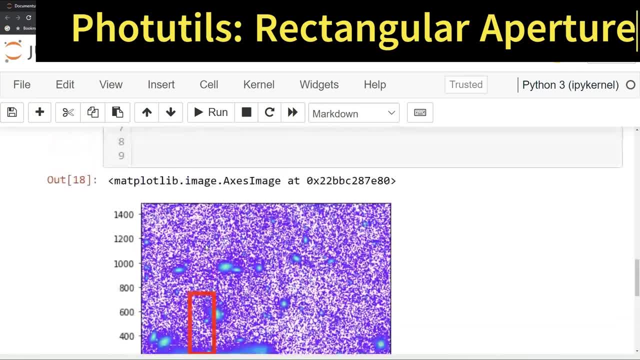 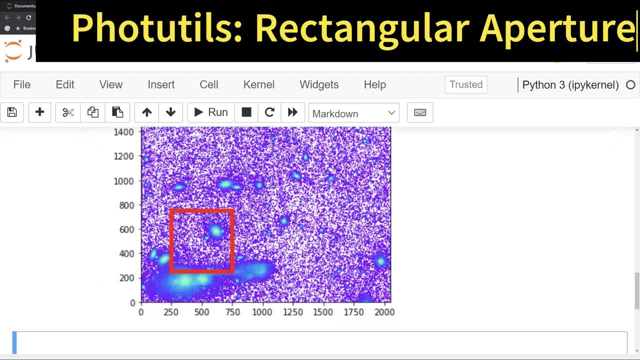 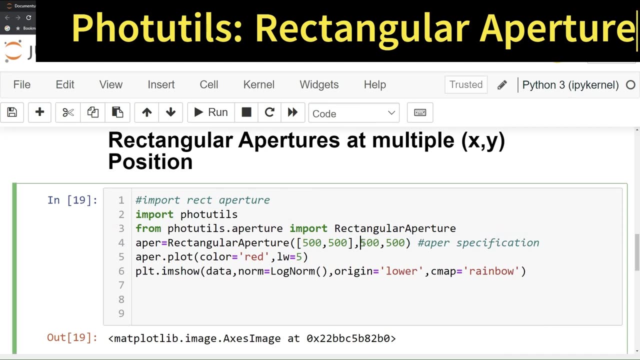 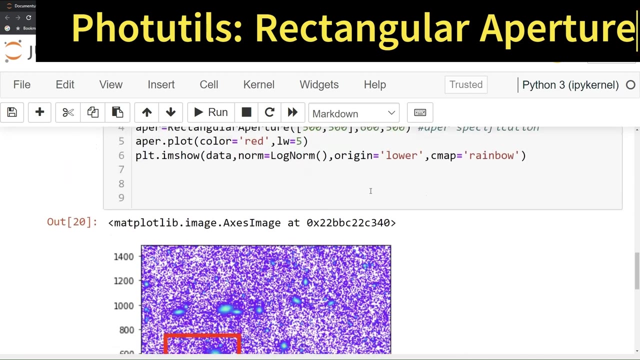 Okay, see, it has increased its width. You can increase, Yeah, Okay. so now it's completely rectangular, So you can also. it's completely a square, So let's make it 600.. So this becomes your rectangular. So if the size becomes same, it becomes a square. Okay, so this way you can do. you can also like plot one more aperture.